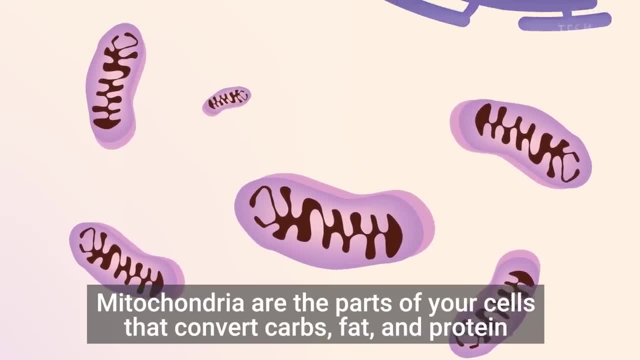 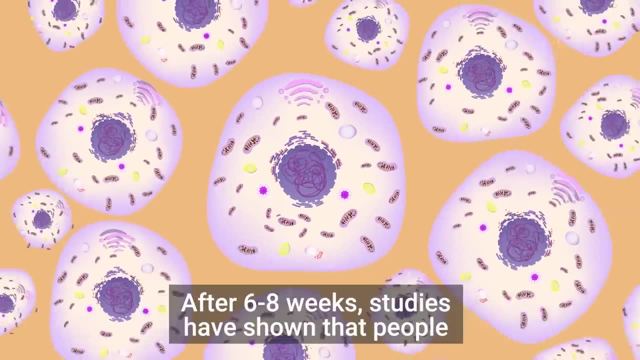 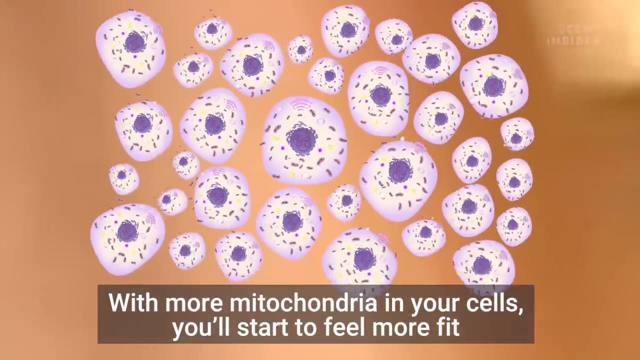 biogenesis. Mitochondria are the parts of your cells that convert carbs, fat and protein into fuel that your muscles use to do their job like flex and contract. After six to eight weeks, studies have shown that people can increase their mitochondria by up to 50%. With more mitochondria in your cells, 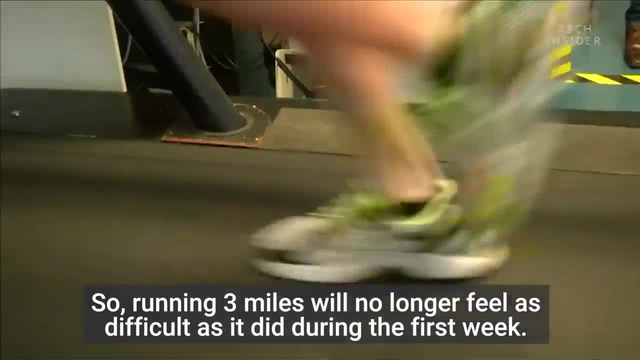 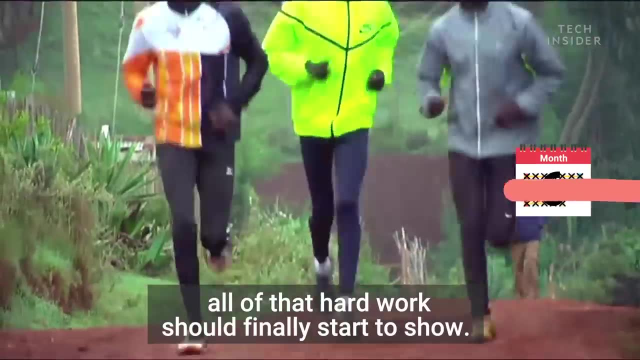 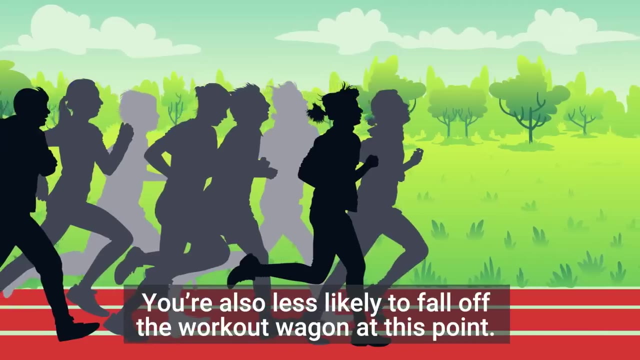 you'll start to feel more fit and your endurance will increase, so running three miles will no longer feel as difficult as it did during the first week. Once you're six months in all of that hard work should finally start to show. If your workouts focus on strength training, you'll notice your muscles begin to take shape. You're also less 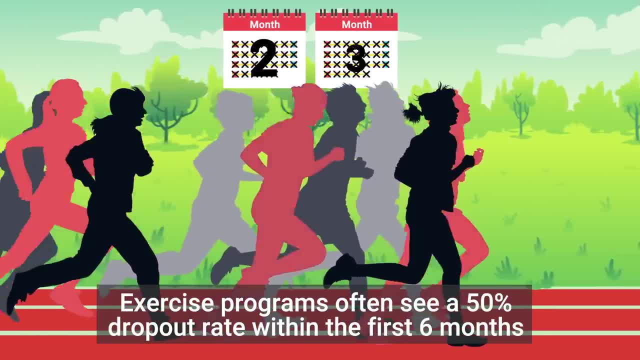 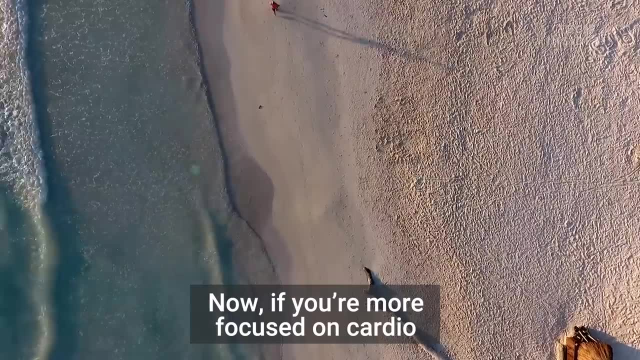 likely to fall off the workout wagon at this point. Exercise programs often see a 50% dropout rate within the first six months, but after that more people stick with it. Now, if you're more focused on cardio, then by nine months of. 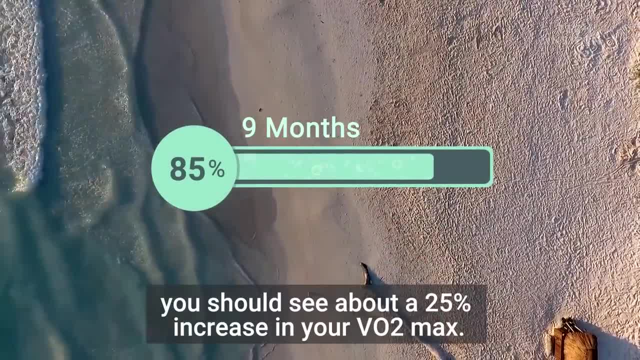 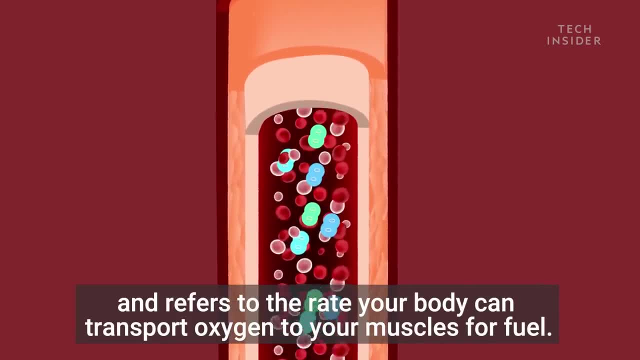 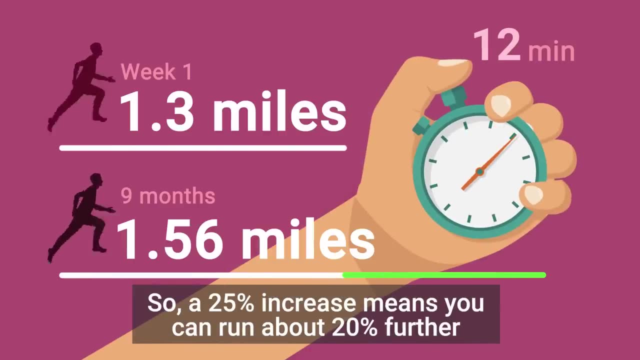 regular exercise, you should see about a 25% increase in your VO2 max. VO2 max is often used as a measure of fitness and refers to the rate your body can transport oxygen to your muscles. Basically, higher VO2 max means you can run faster for longer, so a 25% increase means you can run about 20% further in the same amount of time. 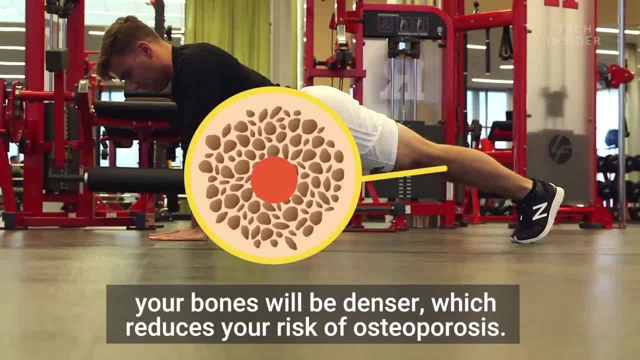 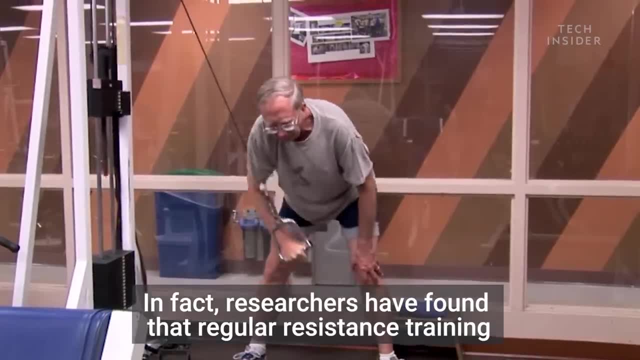 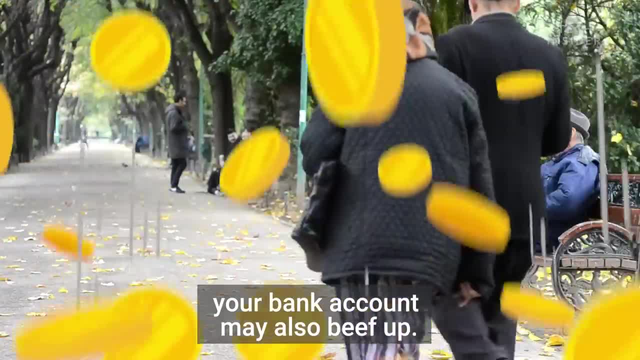 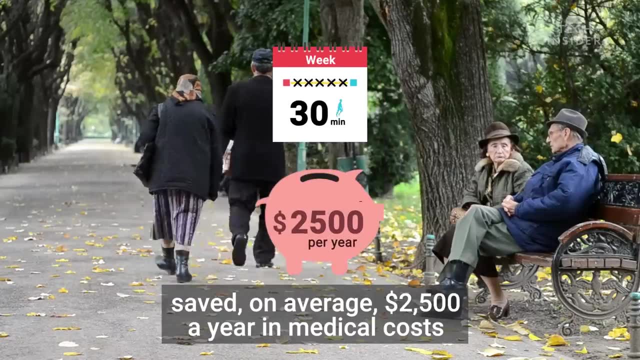 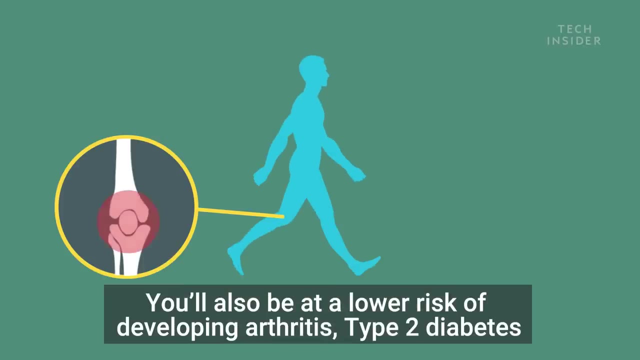 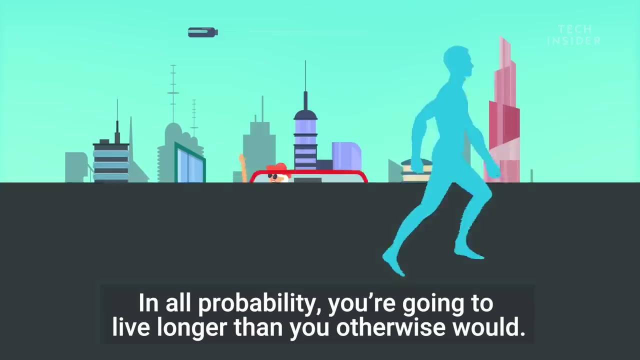